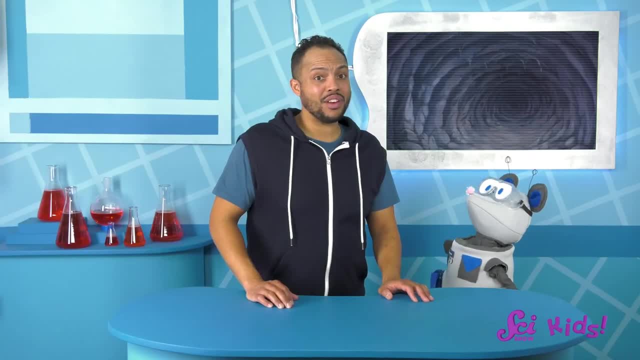 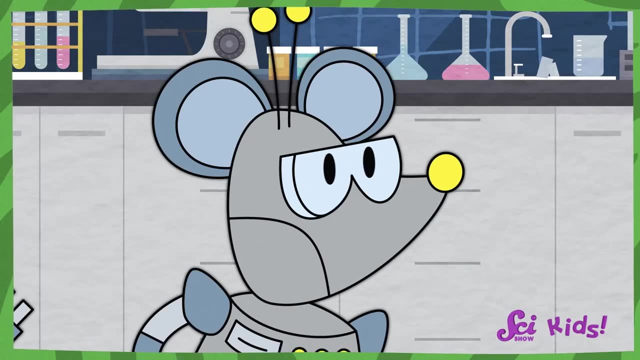 Oh, you're afraid of running into things in the dark. It could be a bit scary trying to get around in the dark if you aren't used to it. Most people use their eyes to help figure out where they're going, and you do too. Squeaks In the dark, you and 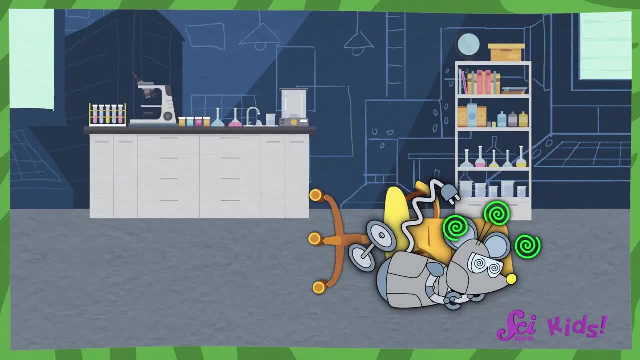 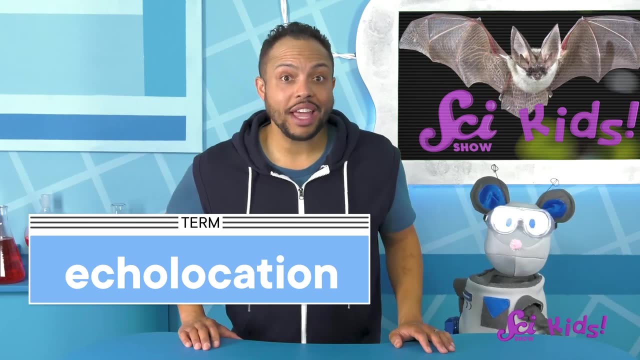 I can't see if there's a wall or chair in our way and we might trip, But Sam and much of his bat family have a special way to help get around their cave safely. Bats can use echolocation. Well, do you know what an echo is? Squeaks. 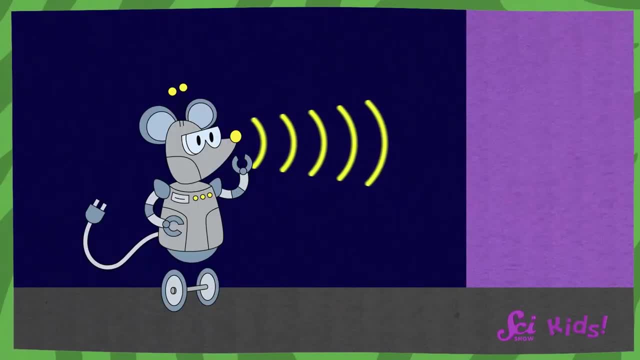 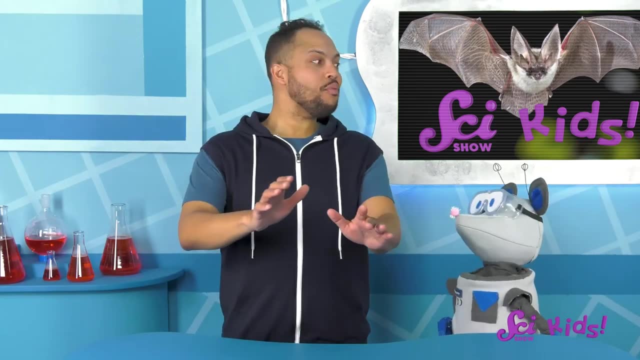 That's right. An echo is when sound bounces off of things and you can hear the sound again and again, Like when you shout in a big room, room, room, room. Echolocation is using echoes to locate or find objects around you, like the walls of. 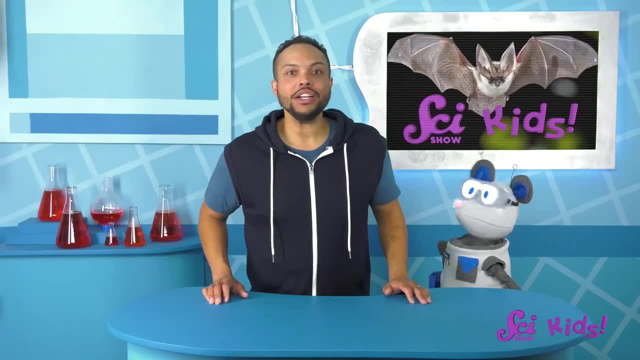 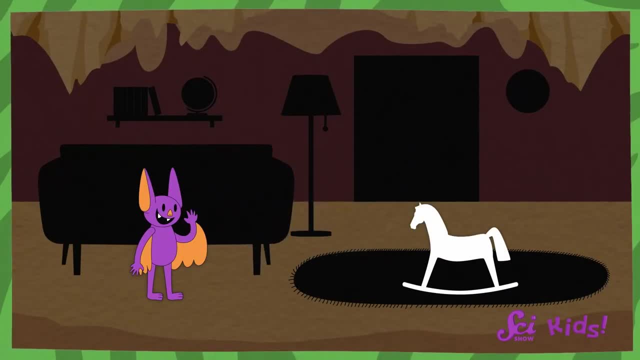 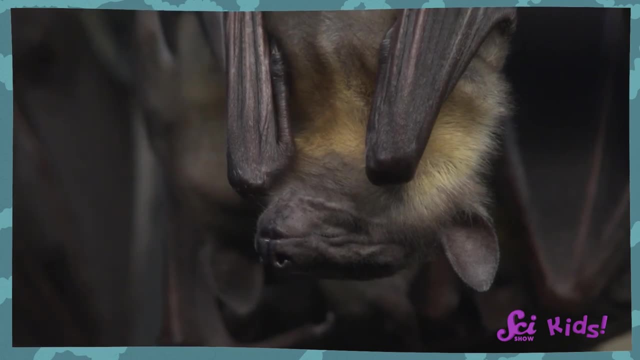 sounds that bounce off of objects. They can make sounds that bounce off of objects. When the sound bounces back to the bat's big ears, the bat can tell how far away the object is and sometimes even what it is. Bats have really big ears so that they can catch a lot of sounds. 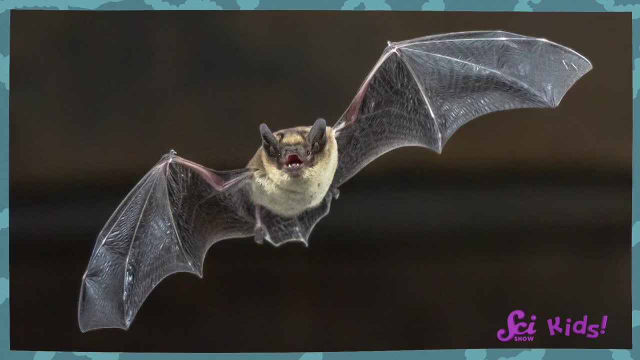 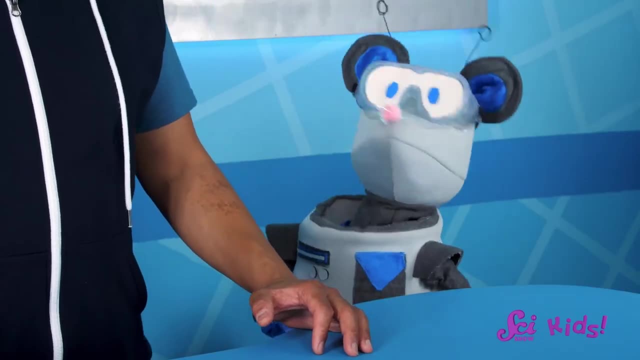 Bats can echolocate to get around in the dark to avoid flying into cave walls or trees outside, And they can also use it to find flying bugs to eat. Echolocation is a pretty amazing skill, and it's not just bats who can do it, Because 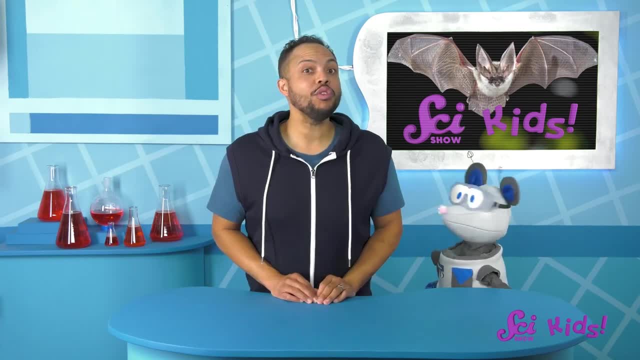 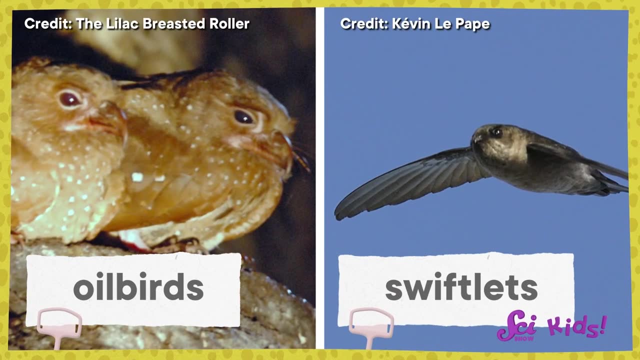 it's so helpful for finding your way in the dark. some other animals who live in dark places can also echolocate. Some birds who live in caves, like oil birds and swiftlets, can echolocate like bats do, And there are other very dark habitats or places that animals live where echolocation. 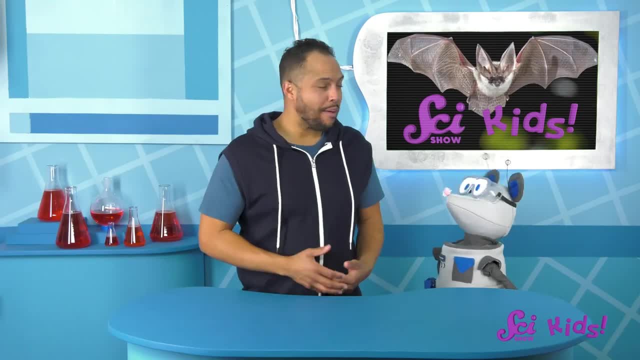 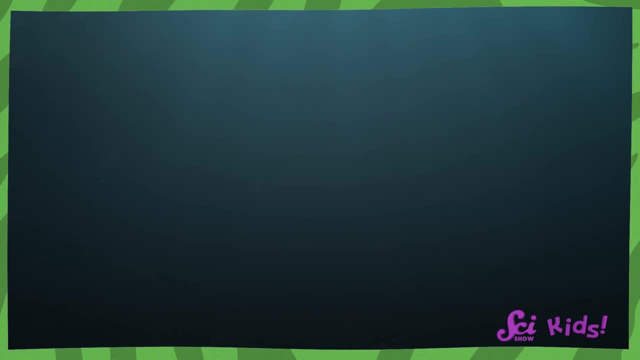 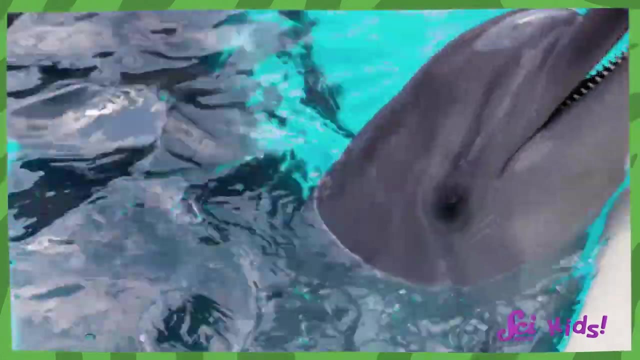 comes in handy Squeaks. can you think of any other habitats that can get really, really dark? The ocean does get super dark below the surface. Some creatures who live in the ocean, like dolphins, can echolocate too. Dolphins are really good at making different sounds.